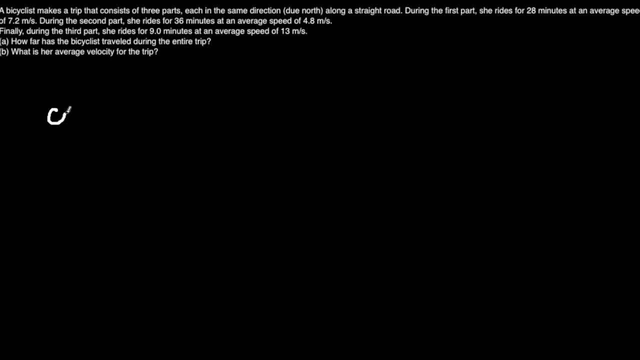 So the first thing that you have to know is the formula for constant speed. For constant speed you only should really have. distance is equal to velocity times time. V can be velocity or speed, It depends on how you will use it, on the context of the problem. 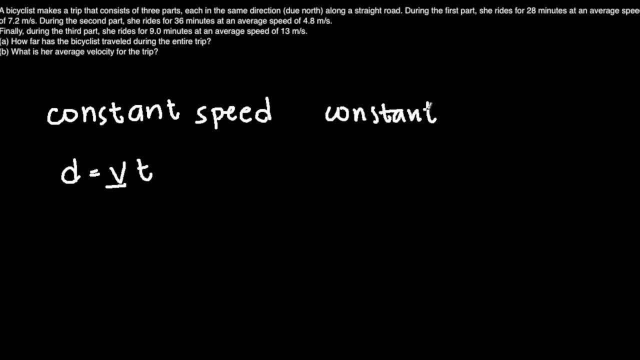 For constant acceleration. I'll give you four formulas that you can use Later on when we start solving the problems. The first formula that you will want to use is: final velocity is equal to initial velocity plus acceleration times time. The second one is the square of the final velocity is equal to the square of the initial velocity plus two times acceleration times distance. 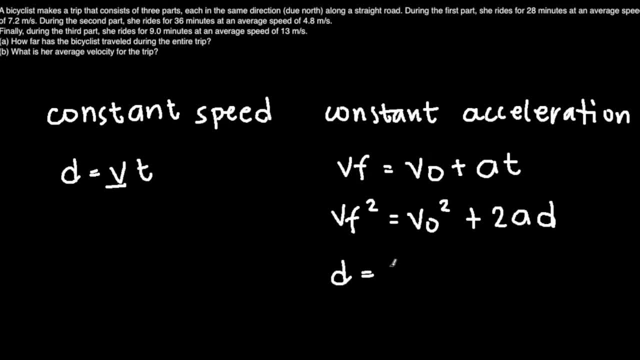 The third one is: distance is equal to one half of The initial velocity plus the final velocity times time. And the last equation that I want you to use for constant acceleration is: distance is equal to initial velocity times time plus one half of the acceleration times time squared. 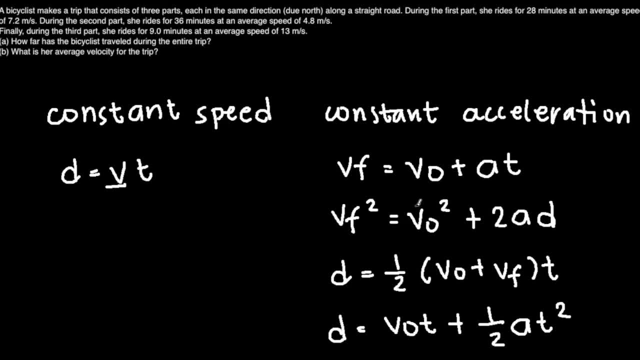 So these are what we call the equations for kinematics. That's what physicists and teachers would call them. So these are what we call the equations for kinematics. So these are what we call the equations for kinematics, Or some books that you might want to read in the future. 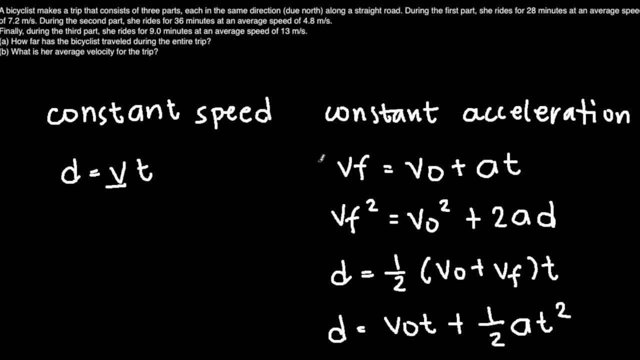 So this is the kinematic equation for constant speed And these are the kinematic equations for constant acceleration. So whenever you read a problem, or whenever a problem talks about constant speed or just doesn't talk about the word acceleration in general, you might want to use the equation for constant speed. 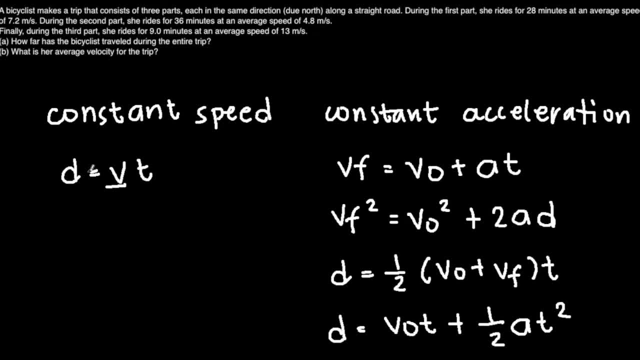 But if the equation or if the problem implies that there is acceleration by telling you that there is final and initial velocity throughout the course of the trip, then you might want to use the four kinematic equations for constant acceleration. So let's start with our very first problem, having the formulas in our mind. 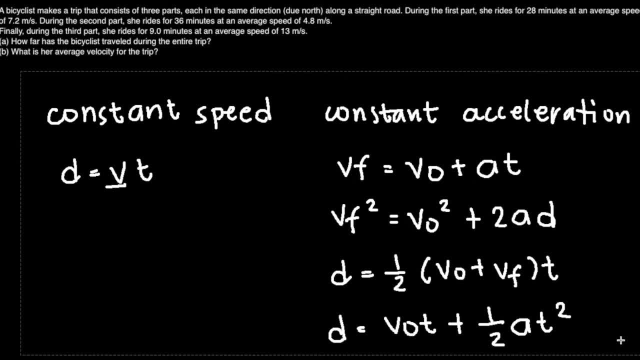 And you might want to write these formulas in your notes, because I want you to memorize them when our quiz and maybe when our exam comes. I want you to memorize them in your mind. so, if ever your notes or the formulas that you've written down in your index cards are incorrect, 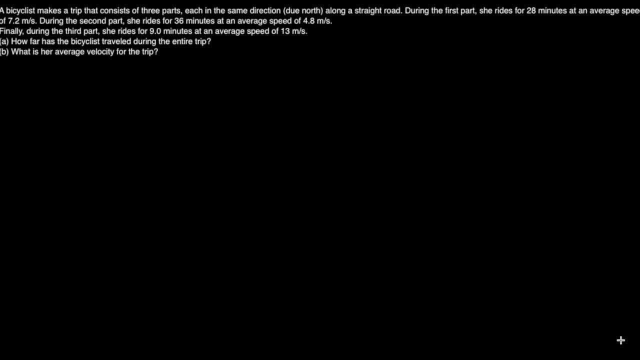 then you always have a backup in your mind. So let's solve the first problem. Problem number one: A bicyclist makes a bicycle And she makes a trip that consists of three parts, each in the same direction, due north along a straight road. 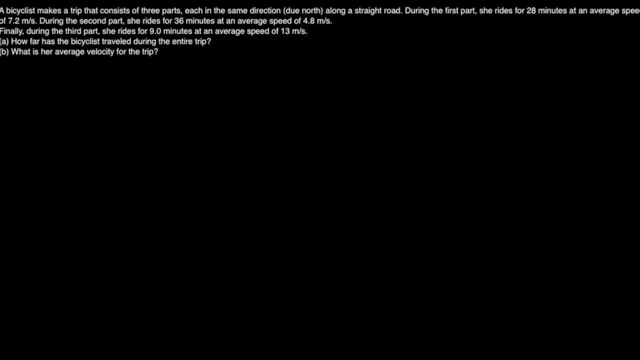 During the first part, she rides for 28 minutes at an average speed of 7.2 metres per second. During the second part, she rides for 36 minutes at an average speed of 4.8 metres per second. Finally, during the third part, she rides for nine minutes at an average speed of 13 metres per second. 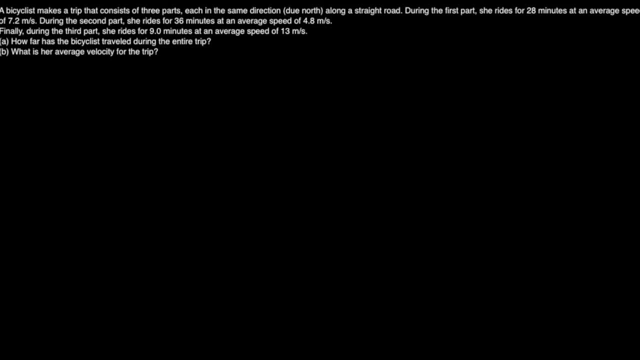 second: A- How far has a bicyclist traveled during the entire trip? And B- What is their average velocity for the trip? So you might notice that we have three segments here. For segment one, the bicyclist is actually traveling to the 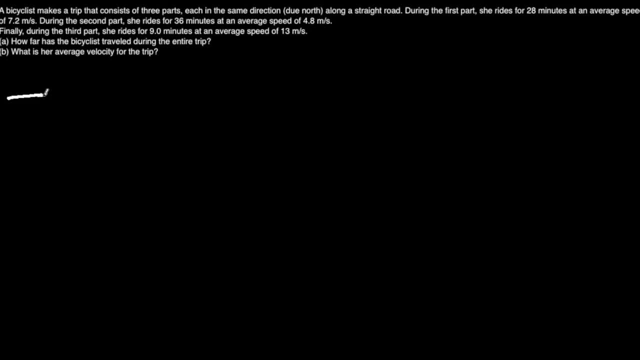 direction of north. so you might want to imagine that this direction that I'm pointing to is not east but north. So this is going to be our north, this is going to be our south, this is going to be our west and this is going to be our. 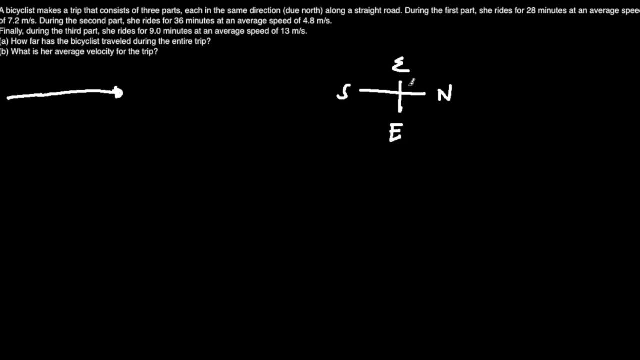 east, So just take that in mind if you're very sensitive with directions. Alright, so let's go back to solving. So during the first part, she rides for 28 minutes at an average speed of 7.2 mps- so you might want to write that down so you won't forget- at 7.2 meters per second. 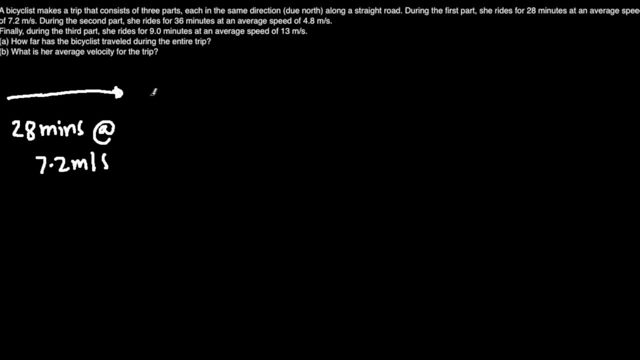 During the second part she's still traveling north. All of her trips are due north, so don't be confused. I'm going to write a line or a vector of the same direction. The second part: she rides for 36 minutes at an average speed of 4.8. 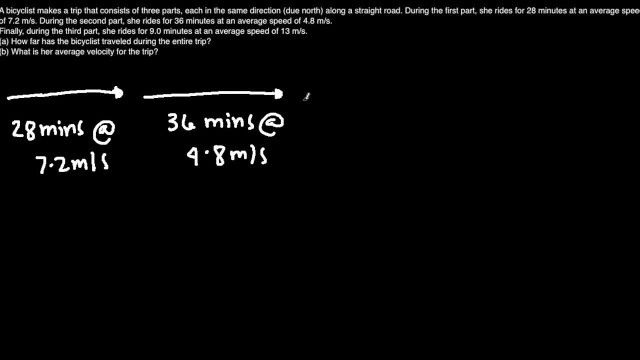 meters per second and she makes a stop or for some reason she changes her speed to 13 meters per second at 9 minutes. So for 9 minutes she travels 13 meters per second at the very last segment or at the very last part. First question is: how far has 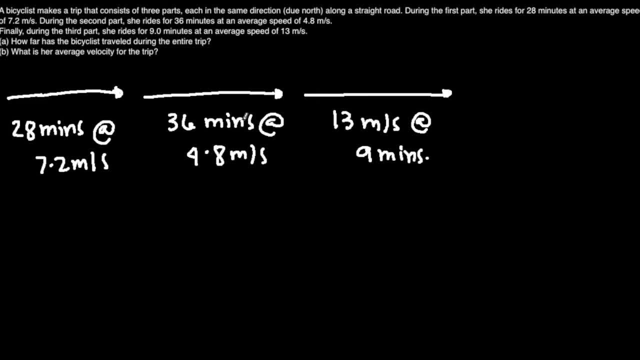 the bicyclist traveled during the entire trip. So this is very simple. We will use distance is equal to velocity times time here, because, yes, the bicyclist is changing her velocity, She's accelerating and decelerating, But we want to get this. 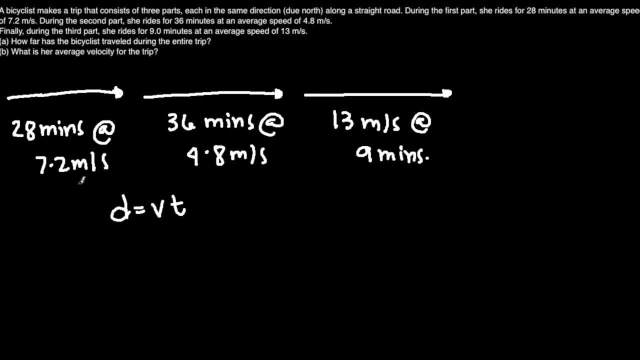 speed ofor we want to get. We already have the speed and the time, but we want to get the distance that the bicyclist has traveled in each of the three segments. So we have segment 1,, segment 2,, segment 3.. 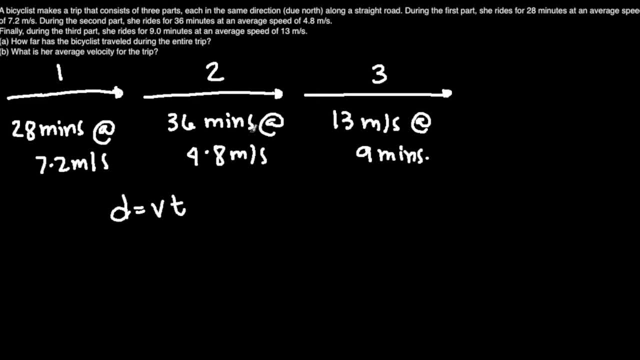 Once we have the individual distance for each segment, then we can add them and then we will have the total distance that the bicyclist has traveled for the entire trip. So let's go for. let's solve for d1.. So d1 is equal to the velocity at the first segment, which is 7.2 meters per second. 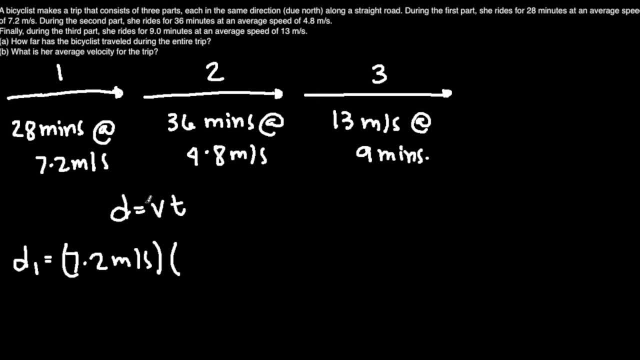 and the time it took for the bicyclist to travel. for the first segment It's 28 minutes. Now you have to be very careful because 28 minutes is in minutes And we would want the unit for time to be uniform. So 28 minutes is approximately 1,680 seconds. 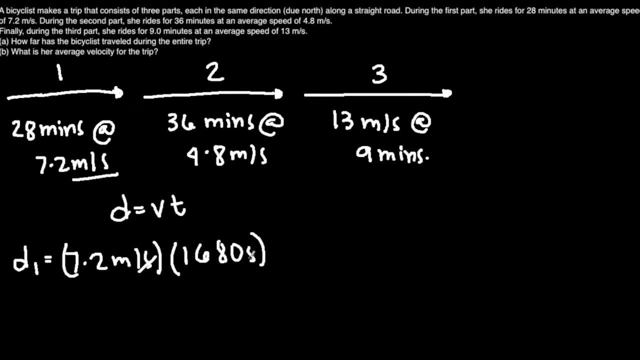 So that's what you would want to write there, So we can cancel seconds once we start solving for the solution and we would only have meters left. So our answer should be in meters, 7.2 times 1,680.. The distance for the first segment should be: 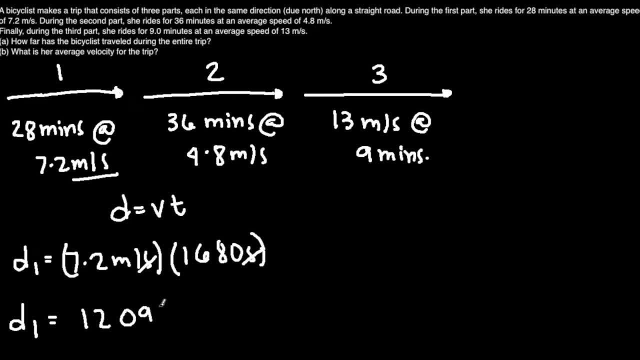 12,096 meters- Very far. I wouldn't walk this distance For our distance 2, then we should just use the quantities available for the second segment. So we do this each part. So let's do this fast. 4.8 velocity. 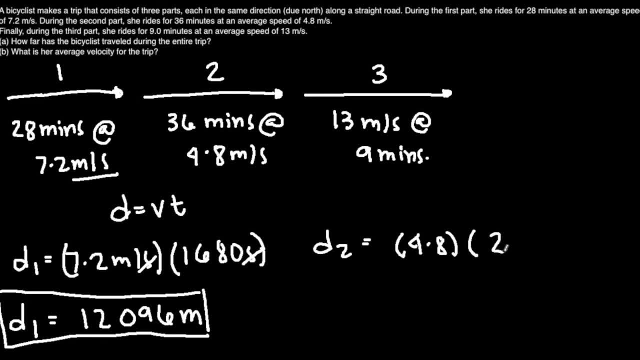 and 36 minutes is 2,160 seconds And if you try to calculate, you have 10,368 meters. for the second distance And for distance 3, let me see if I can put it here. For distance 3, we have 13,, which is the velocity. 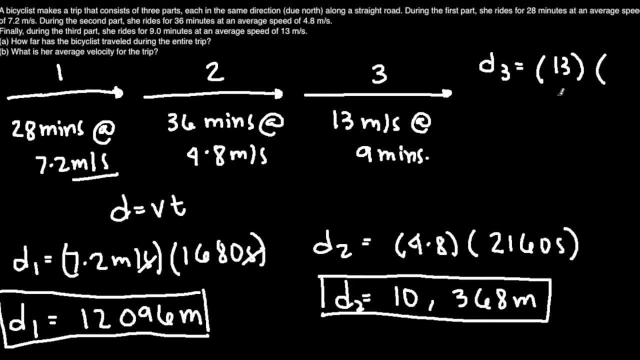 times 9 minutes in seconds is 540.. So distance 3, you have approximately 7,020 meters, Or these are the individual distances that the bicyclist has traveled in each individual segment. So if you want to get the total, let's say: 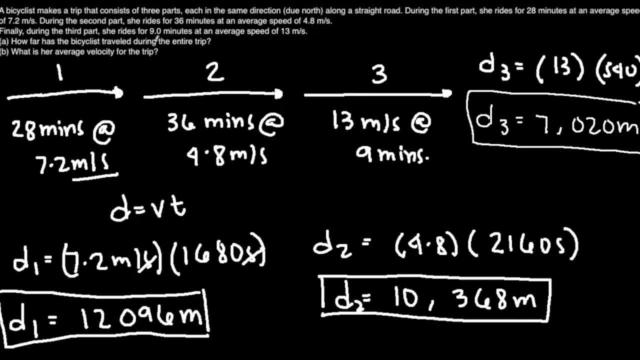 the total distance that the bicyclist has traveled during the entire trip. so we just have to add everything. So if you want to add distance 1, plus distance 2, plus distance 3,, the total distance would be 29,484 meters. 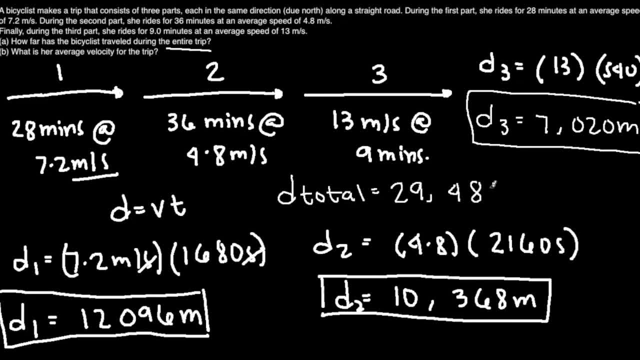 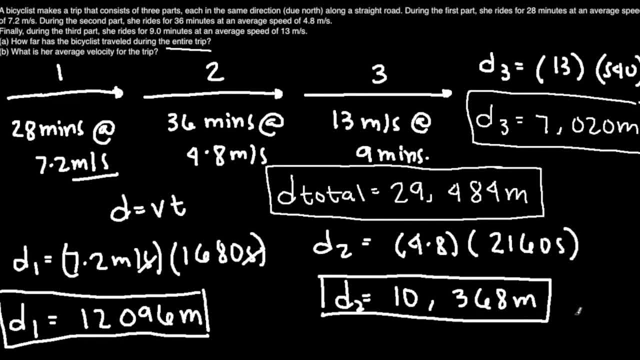 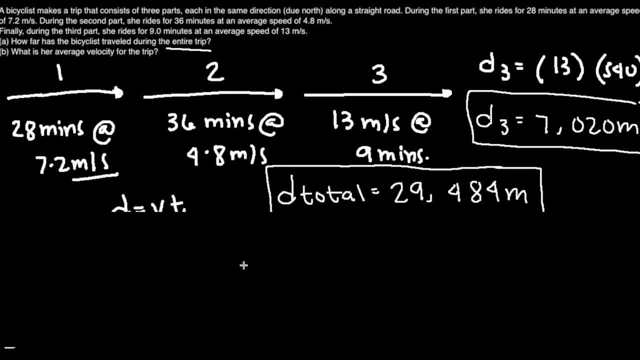 Letter B: What is your average velocity for the trip? So let me just clear some space, because I need some space here. Okay, So the average velocity is equal to the total distance or displacement traveled over the total time We have. We already calculated our total distance, which is 29,484 meters. 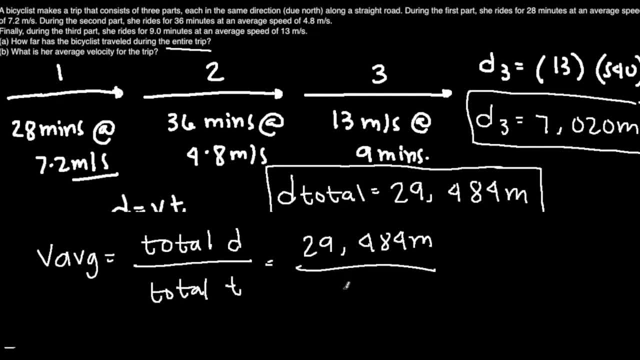 And we also did calculate for the total time, But you have to add up all the individual time in seconds. Okay, So if you try to add everything up, we have 4,380 seconds. 4,380 seconds is from the individual: 28 minutes, 36 minutes and 9 minutes in seconds. 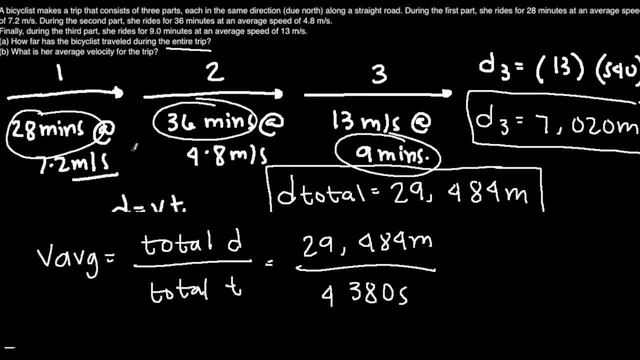 So you just want to convert the minutes to seconds, Add everything And then you will come up with 4,380 seconds, which is the total time it took for the bicyclist to travel the entire trip. So average velocity- if you try to compute, it is going to be 6.73 meters per second. 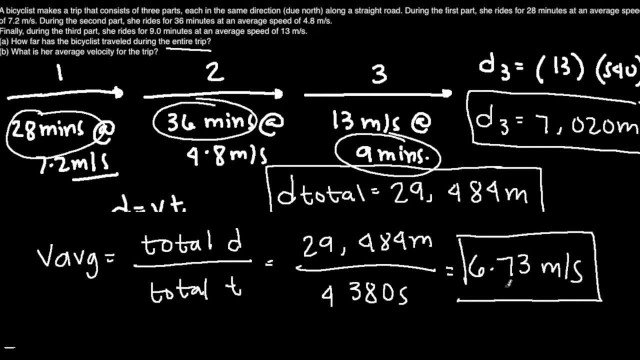 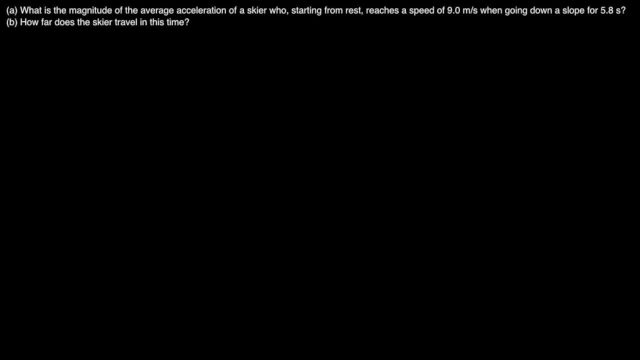 So that's our answer for letter B. What is the magnitude of the average acceleration of a skier who, starting from rest, reaches a speed of 9.0 meters per second when going down a slope for 5.8 seconds? And letter B: how far does the skier travel in this time? 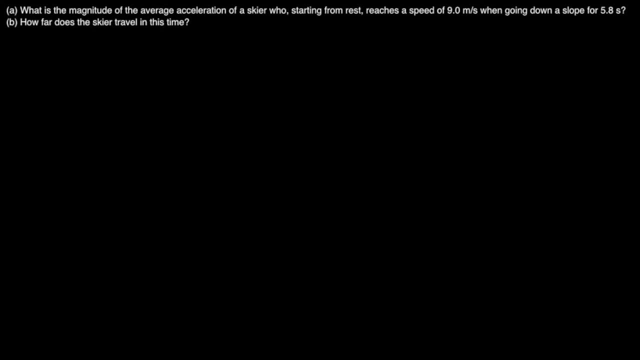 So for the first part, we have to get the acceleration of the skier. The quantities that we are given are The initial velocity. of course, The initial velocity should be 0 meters per second, because it literally said: starting from rest. Whenever you hear or whenever you read in a problem from rest, that means the initial velocity is 0 because it's resting. obviously. 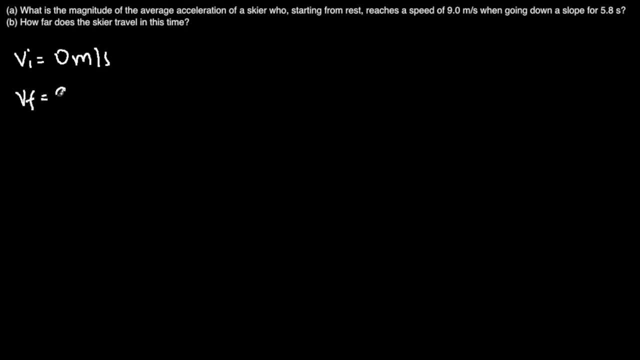 You also have the final velocity, which is 9.0 meters per second, Because if you try to read it, it reaches a speed of 9.0 meters per second. When you reach something, that means that's implied as your final velocity, because you've already reached it. 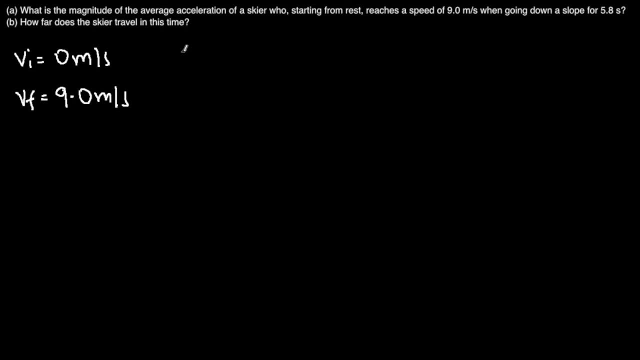 And we also have the time. so everything happened for 5.8 seconds. And then we want to get the acceleration. Which kinematic formula has all of the initial velocity, Final velocity, the time and the acceleration in it? So I want you to pause the video and try to find the perfect formula that best suits in solving the acceleration. 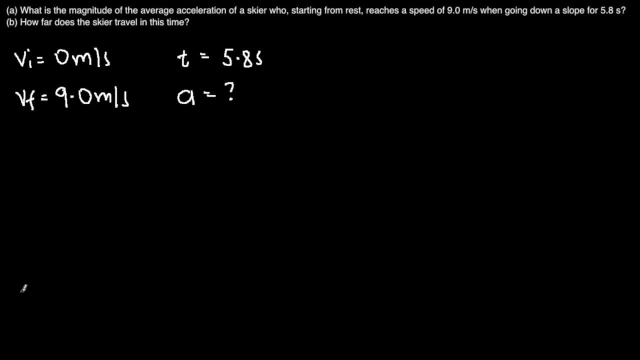 So it turns out that the formula that we need is: Final velocity is equal to initial velocity plus acceleration times time. So So we just have to substitute the quantities into the variables, So we have 9.. You don't really have to write the units anymore. 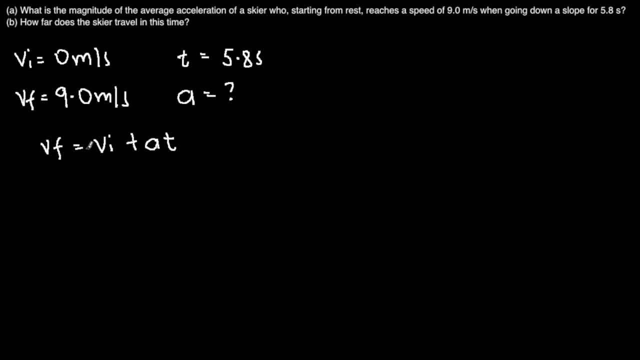 Just make sure that before you plug it in in your formula, that all of your units are uniform. So you have seconds for time, for velocity or for speed. Your unit for time should also be seconds, And then meters in here, And then meters in everything. 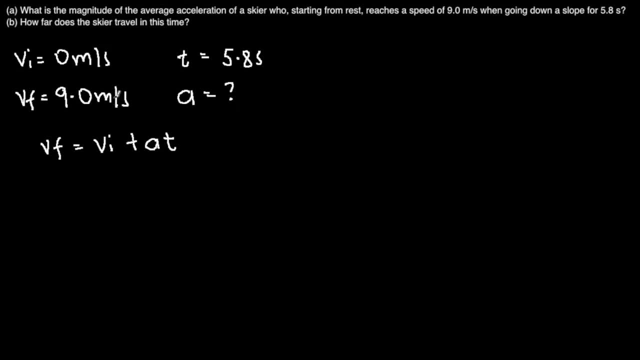 So I think we're good to go for the quantities and for the units. So we just have to plug it in. So we have: 9 is equal to Your initial velocity is 0. anyway, If you have anything that is 0, please don't write it anymore. 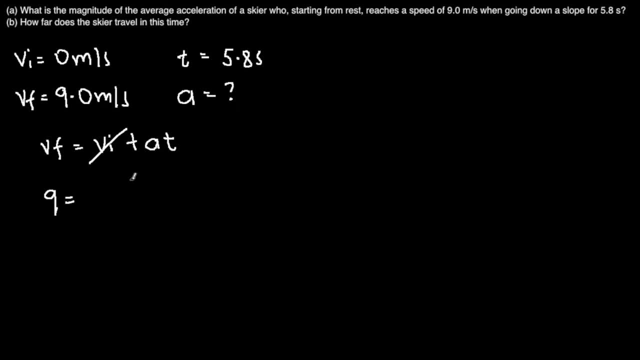 Just lash it out and then continue with the next term. So we just really have a t for the second or for the right part of our equation. For the time you have 5 points. For the time you have 5.8 seconds. 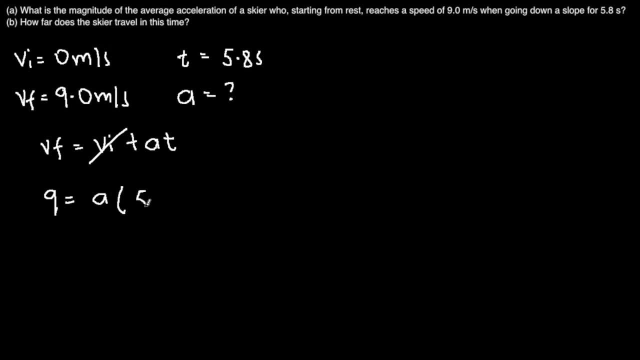 So let's plug it in there. So we have 5.8.. In order to find the acceleration, let's divide both sides of the equation by 5.8.. So you have 5.8 and then 5.8.. 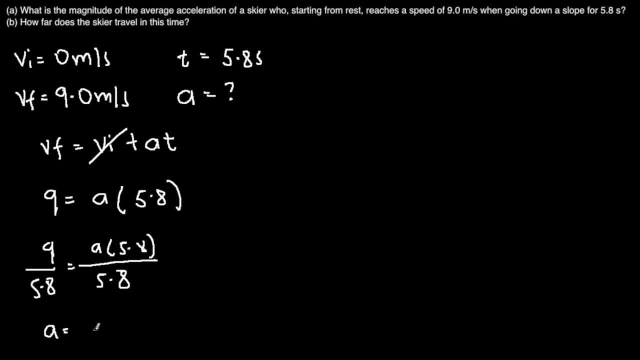 This is 9.. Acceleration should be equal to 1.55 meters per second squared. Please, please, get your units right, because even if your numerical value is correct and your unit is incorrect, then your final answer will be incorrect. So your acceleration should be: 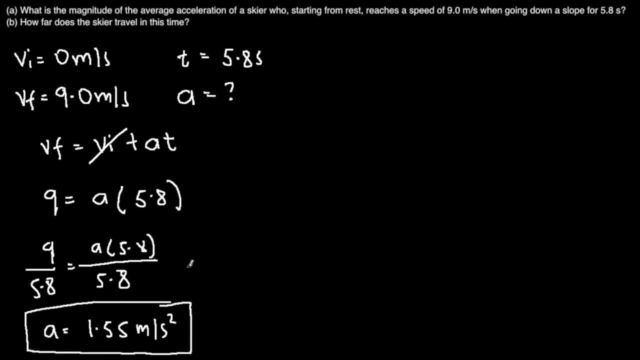 1.55 meters per second, squared For letter B. how far does this gear travel in this time? So we're looking for the distance, that's the skier has traveled in this setup. So what kinematic equation do you think should we use? 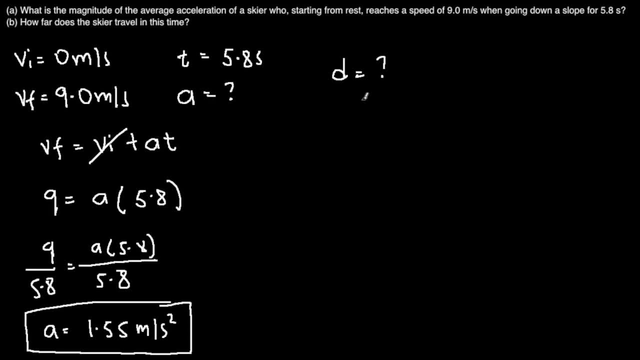 Remember that this problem involves acceleration, So please don't ever use d is equal to vt, because that's for constant speed. So if your problem suggests that it has constant acceleration, just please choose among The kinematic equations for constant acceleration for any of the quantities that you might want to find. 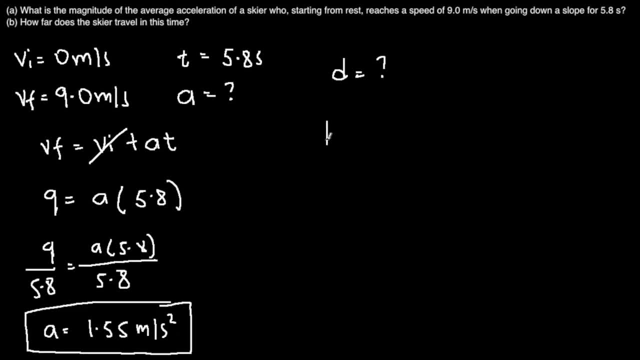 So for distance we just have to use: d is equal to 1.5 of acceleration times time. This formula is from: d is equal to vot plus 1.5 at, but our initial velocity is 0. So we just have to slush this out. 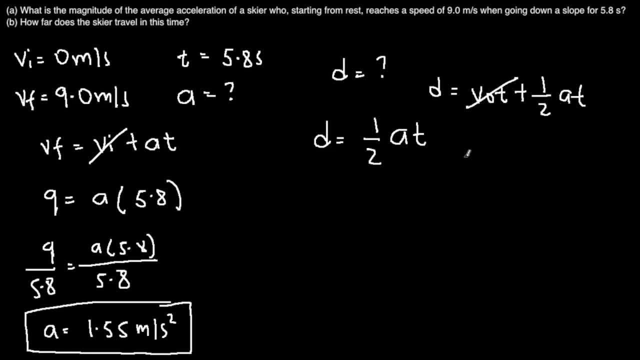 So all we really left is 1.5 at. So let's try to plug our variables in or our values in. Acceleration is 1.55 and then our time is 5.8.. So distance is equal to 4.50 meters. 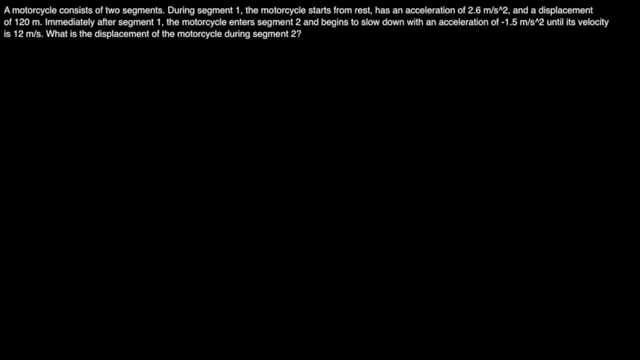 So that's it for this problem. Problem number three: A motorcycle consists of two segments. During segment one, the motorcycle starts from rest, has an acceleration of 2.6 meters per second squared and a displacement of 120 meters Immediately after segment one. 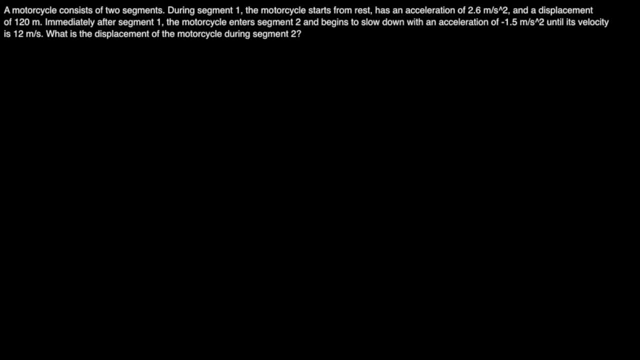 the motorcycle enters segment two and begins to slow down with an acceleration of negative 1.5 meters per second, squared, until its velocity is 12 meters per second. What is the displacement of the motorcycle during segment two? So we have two segments in this problem. 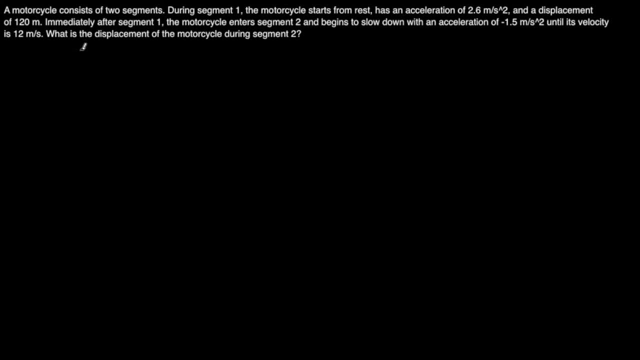 We have to dissect the problem first, in order for us to find the displacement on segment number two. For segment number one, let me write a roman numeral one. our initial velocity should be 0. Because if you try to read here, the motorcycle starts from rest. 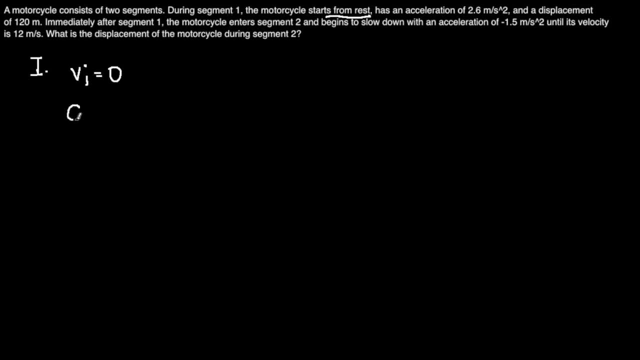 during segment one. Its acceleration is equal to 2.6 meters per second squared And its displacement is equal to 120 meters. After that, the information on segment two is given. The motorcycle enters segment two and begins to slow down with an acceleration. 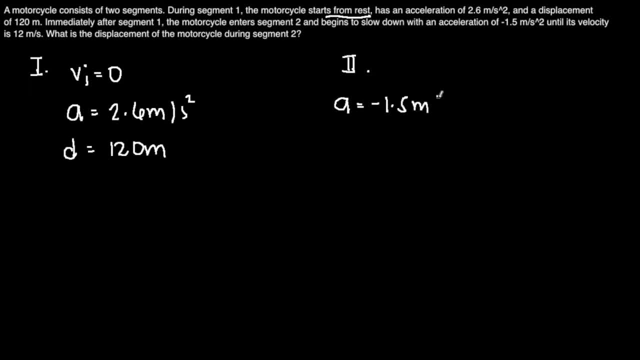 of negative 1.5 meters per second, squared Until its velocity, is 12 meters. Notice that it said until its velocity, So that should give you an idea that that's its final velocity. So 12 meters per second is your final velocity. 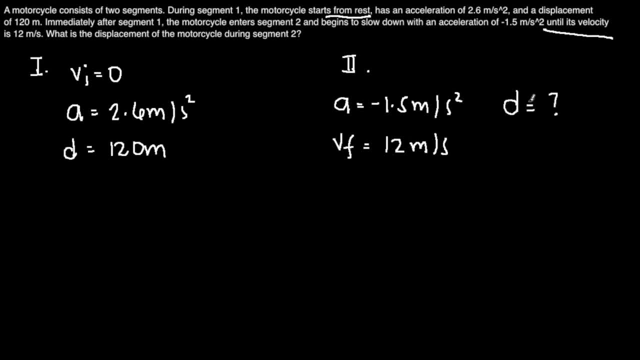 The question is: what is the displacement on the second segment? Now for the second segment, we can use the formula final velocity squared equal to initial velocity squared plus 2ad. We have final velocity which is 12.. We have the acceleration, which is negative 1.5.. 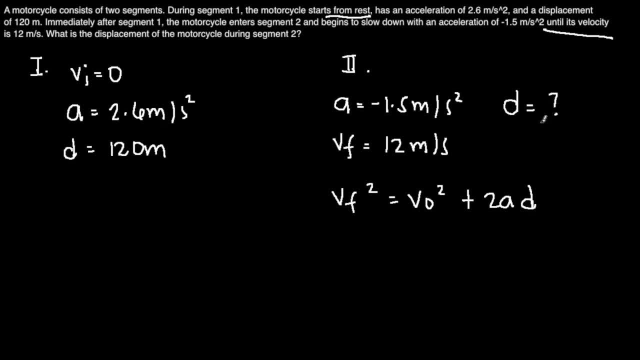 And the distance is what we're looking for, But we're missing one variable, which is our initial velocity in segment number two. A value for the third variable, which is the initial velocity on segment number two, can be obtained by noting that it is also the final velocity. 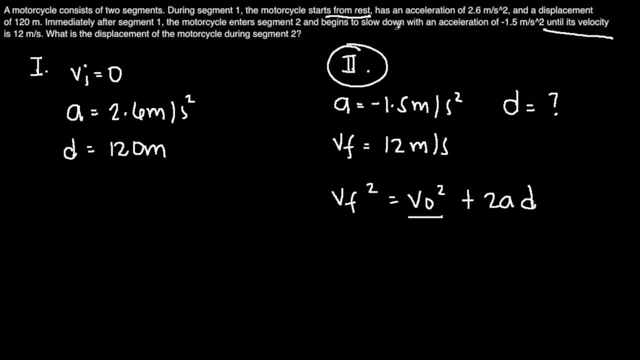 of segment number one. So as the motorcycle leaves segment number one, it has a final velocity right. So when it enters segment number two, the final velocity of segment number one is the initial velocity for segment number two, And that's what we will plug in here. 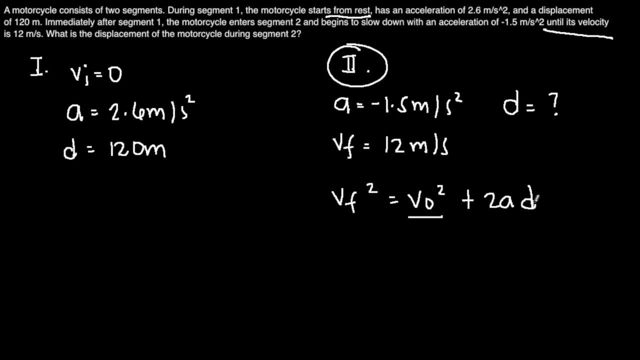 so we can find the distance. But how do we find the initial velocity on segment number two? We just simply find the final velocity in segment number one. So for segment number one, in finding the final velocity we can use the same formula. 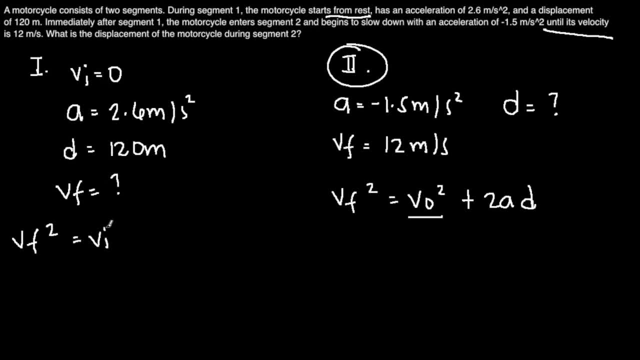 which is vf squared is equal to vi squared plus 2ad. Make sure that all of your units are uniform and consistent And after making sure, just plug in the numbers So you have. vf squared is equal to 2 times 2.6. 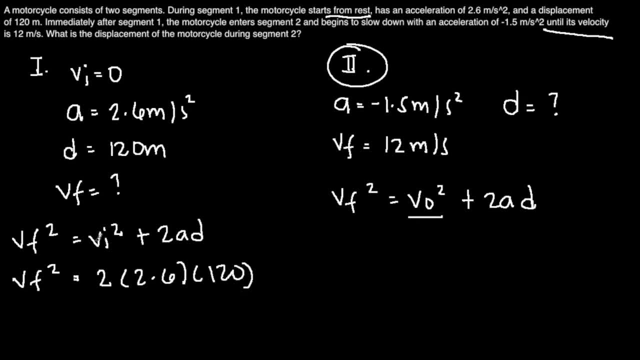 times 120.. You might notice that I didn't put anything for the initial velocity, since our initial velocity for segment number one is zero, So let's just lash it out And we are left with this term. So 2 times the acceleration times the distance. 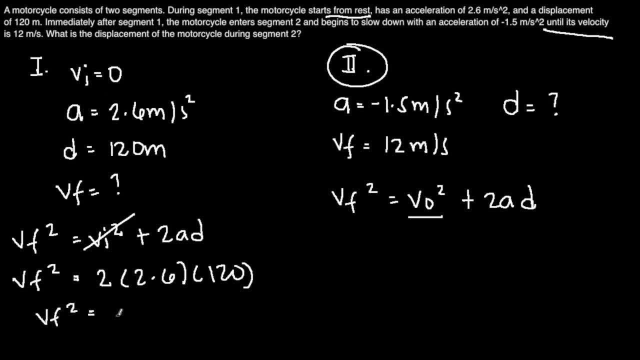 So our vf squared is equal to 624.. Take the square root of both sides of the equation and then we have: vf is equal to 24.98 meters per second. This is the final velocity for segment number one And as soon as it enters, 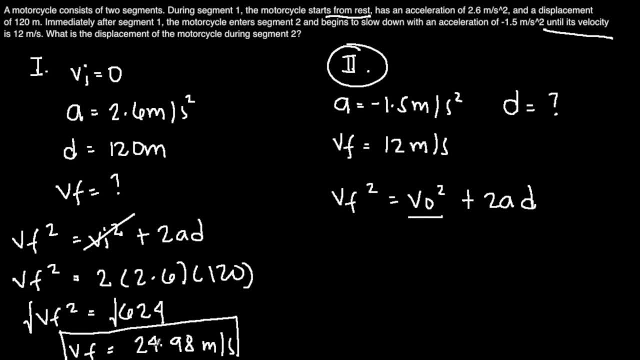 the second segment, the final velocity will be its initial velocity, So let's write that down here. Our initial velocity is 24.98 meters per second. Now we can solve for the distance because we already have the initial velocity for the second segment. 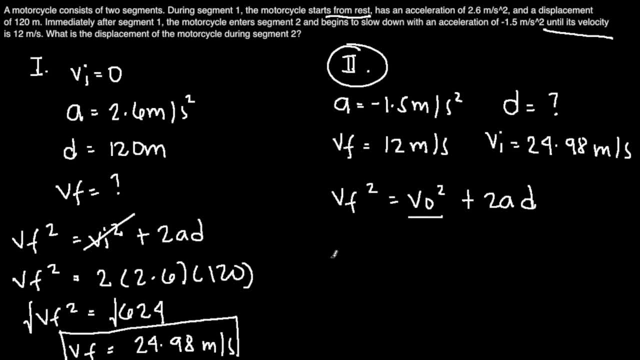 So let's plug in all the quantities that we have. We have 12 squared for the final velocity is equal to 24.98 squared plus 2, and then negative 1.5, and then right distance Square of 12 is 144.. 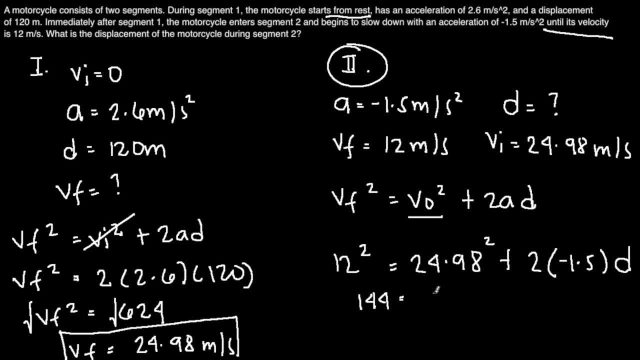 The square of 24.28 is 624.. Plus 2 times negative 1.5 is negative 3.. So let's just put negative 3d there. So we really have transpose 624 to the left side of the equation and we will be left with 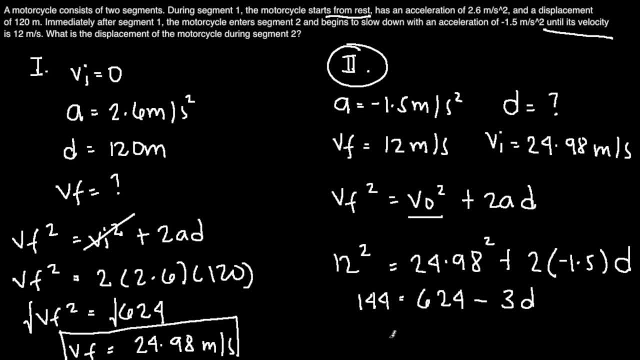 624 minus 624. for the left side of the equation We have negative 480.. And then for the right side of the equation, we are left with negative 3d. Divide both sides of the equation by negative 3.. So d is equal to. 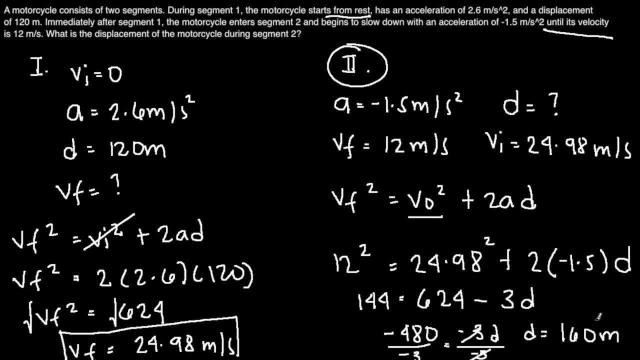 160 meters. So let's just put a box on top of that. So the distance for, or the displacement for, segment 2 of the motorcycle is 160 meters. Very simple, And that's it for this problem. Let's move on to the next problem. 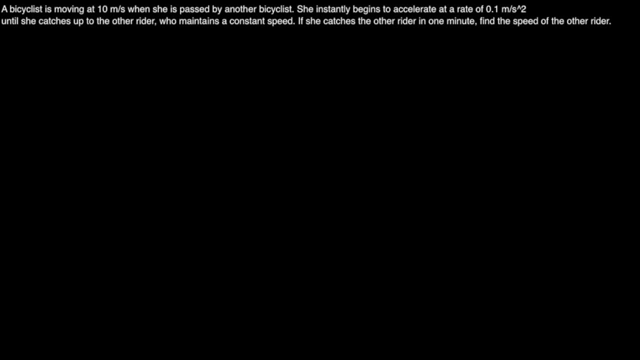 Problem number 4.. A bicyclist is moving at 10 meters per second. when she is passed by another bicyclist, She instantly begins to accelerate at a rate of 0.1 meters per second until she catches up to the other rider who maintains a constant speed. 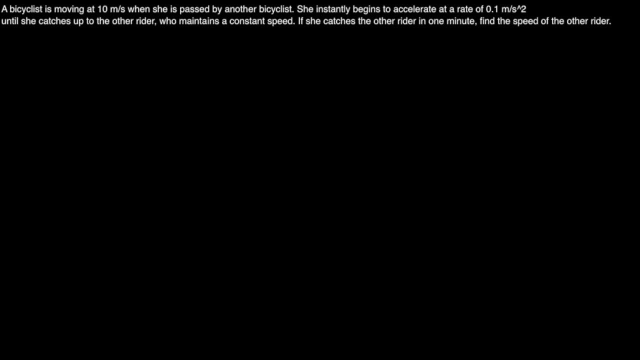 If she catches the other rider in one minute, find the speed of the other rider. So let's try to label and take this slowly because it really needs analysis. So we have bicyclist number 1. Let's write b1 and then b2. 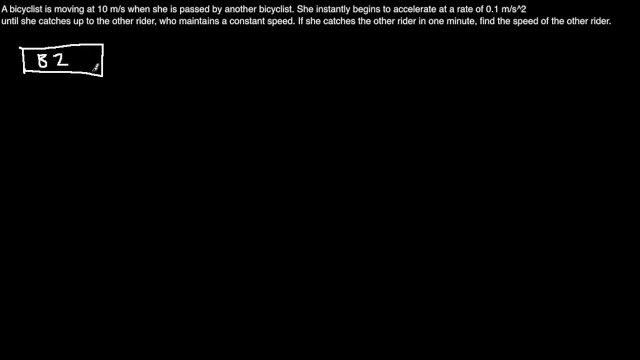 just like the bananas. So bicyclist number 1 is just minding her own business, and she initially has a speed of 10 meters per second, And then here comes bicyclist number 2 who goes past her. So let's see bicyclist number 2. 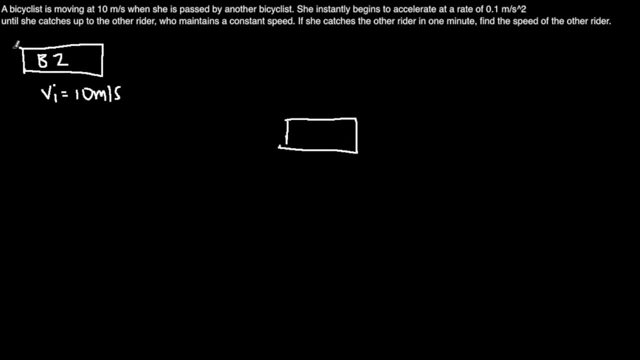 is here. I'm sorry, This should be bicyclist number 1.. I made a mistake. Bicyclist number 1 and this is bicyclist number 2, who just moved past her. So bicyclist number 1 seems very competitive. 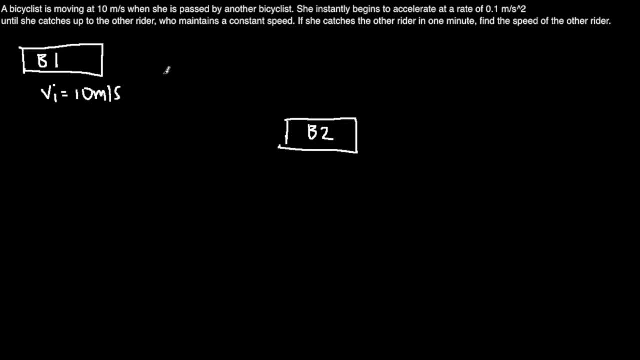 So she tried to accelerate to catch up to bicyclist number 2.. So she tries to accelerate to catch up with an acceleration of 0.1 meters per second squared, And it says here, furthermore, that she catches the other rider in one minute. 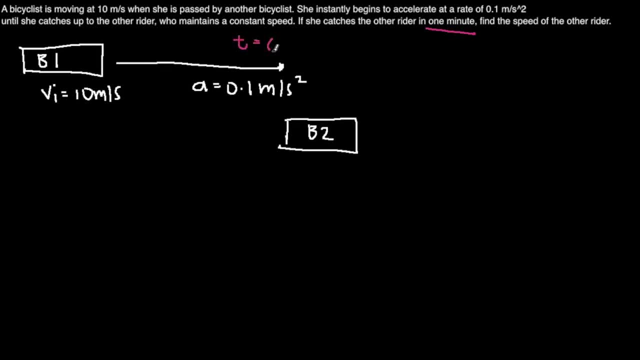 So after one minute, time is equal to 60 seconds. Both bicyclists are at the same distance, So let's just save that after 60 seconds they're both at the same time. I mean at the same distance or displacement. So we have to find 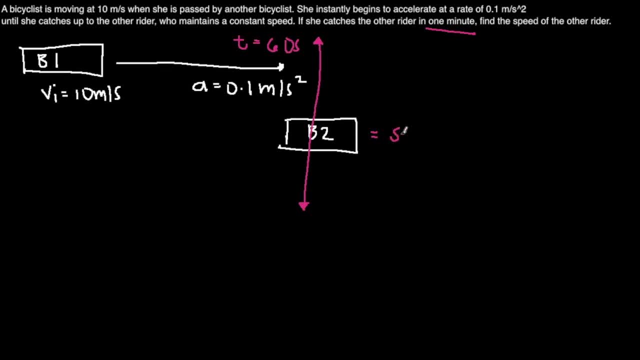 B2's speed. So speed of bicyclist number 2 is what we're looking for. The secret here is to find the distance or displacement of bicyclist number 1 after 60 seconds. So for bicyclist number 1, the given we have our initial velocity. 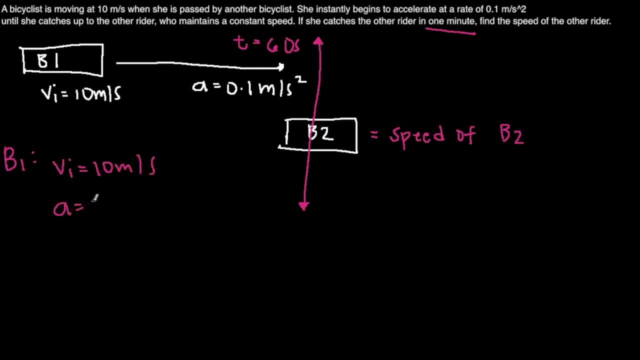 is 10 meters per second, Acceleration is 0.1 meters per second squared And the time is 60 seconds, because that's equal to one minute. So we want to find the displacement of B1, or bicyclist number 1, after. 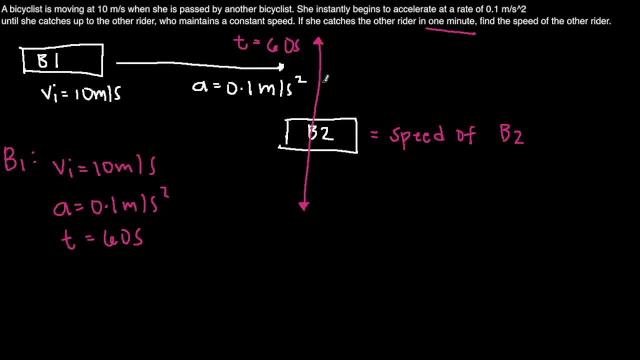 60 seconds And also at that displacement they're equal to each other, Because after 60 seconds they already caught up with each other. So that means they should be at the same displacement after 60 seconds. So we want to find B1's displacement. 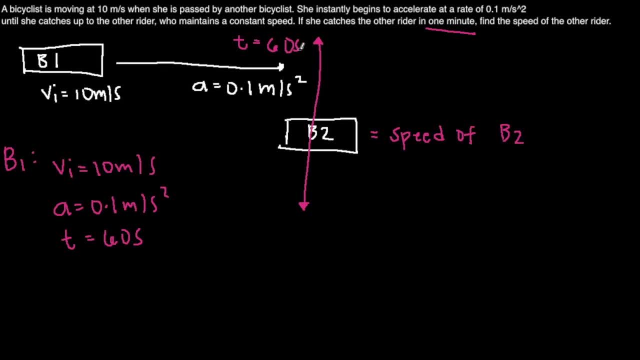 after 60 seconds, because that's also the same displacement with B2 after 60 seconds. So if we try to write it, that's displacement, the displacement that both have after 60 seconds. So how can we find B1's displacement after 60 seconds? 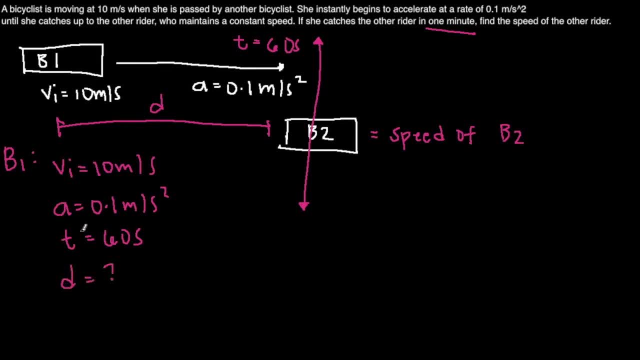 if we have the initial velocity, the acceleration and the time, It turns out that we can use this formula: distance is equal to initial velocity times time plus one half of the acceleration times squared. We have initial velocity, we have the time, we have the acceleration and we also 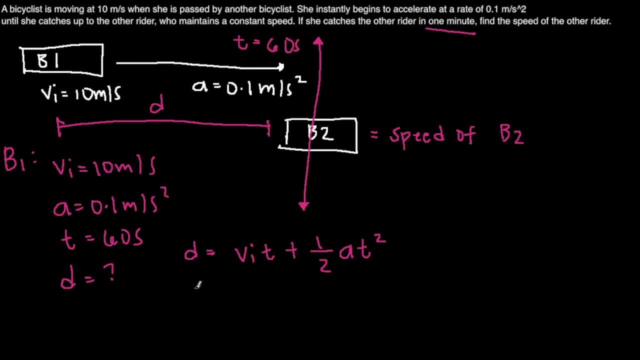 have the time, So let's just plug it in. Let's plug in all the values, So we have: D is equal to 10 times 60 plus one half of 0.1 times 60 squared. So let's use our calculator. 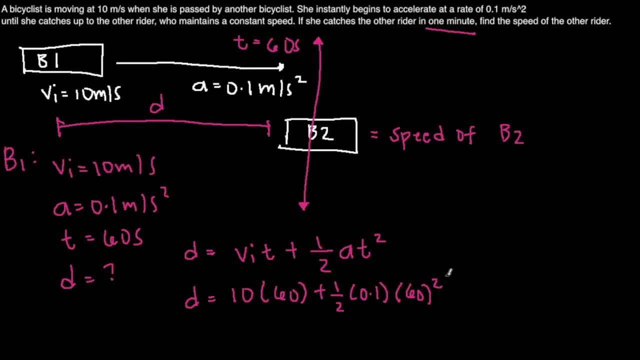 to calculate that. So we have 780 meters for the distance. so at 780 meters they already are at the same displacement because they already caught up. She catches the other rider in one minute. So after one minute, which is a displacement of 780. 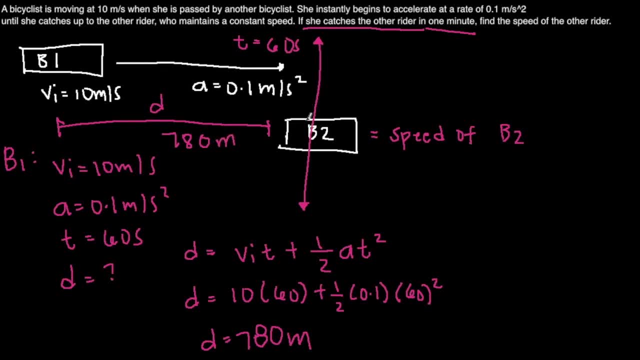 meters. they should be both at the same distance from the initial point, And that's 780 meters. That should also be the displacement of the second bicyclist after 60 seconds. So, in order for us to find the velocity or the speed of the second bicyclist, we 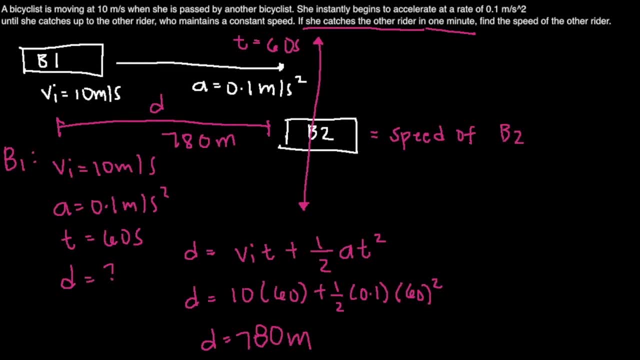 have to use the formula. let's use another color we have to use the formula. D is equal to Vt. Why? Because take note that the second bicyclist is just maintaining a constant speed and whenever we have a constant speed, we just use this one. 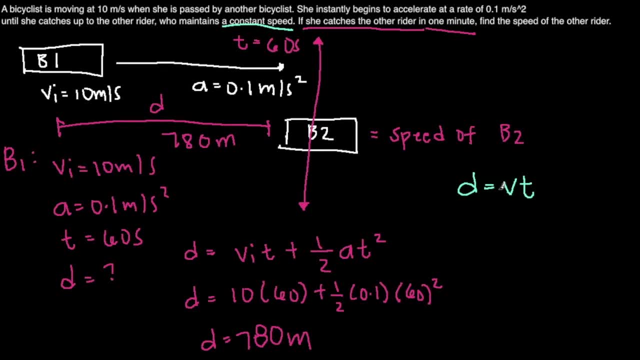 So if we try to find the velocity or the speed from this formula, it's just: V is equal to distance over time. The distance of the second bicyclist is 780, and the time it took for the second bicyclist to go to 780 meters is also. 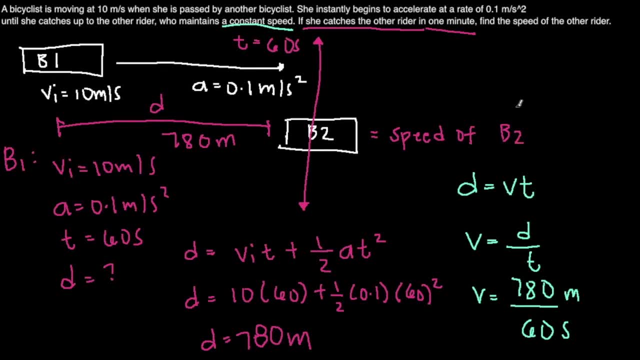 60 seconds. So our velocity should be 13 meters per second. squared I mean 13 meters per second if I put that correctly in my calculator. So let's just verify. It's 13 meters per second. The speed of the second bicyclist. 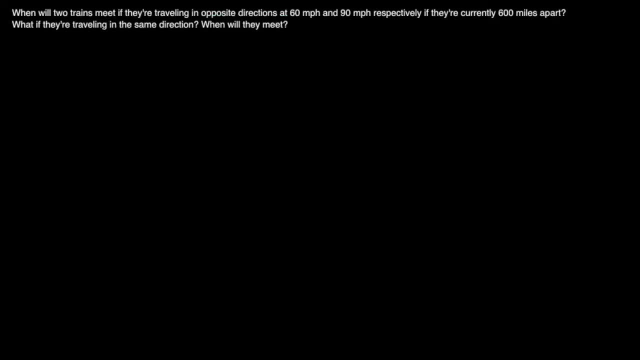 is 13 meters per second. When will two trains meet if they're traveling in opposite directions at 60 miles per hour and 90 miles per hour respectively, if they're currently 600 miles apart? And what if they're traveling in the same direction? When will? 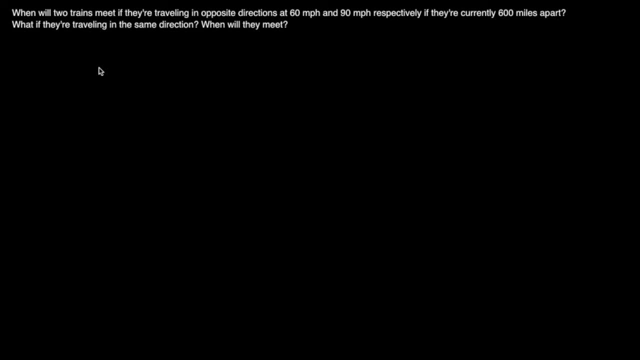 they meet. So the first thing that I'd like to do in this problem is to draw what I have. So the first thing that I have is a train, and they're traveling in the opposite direction. So we have train 1, T1 and then 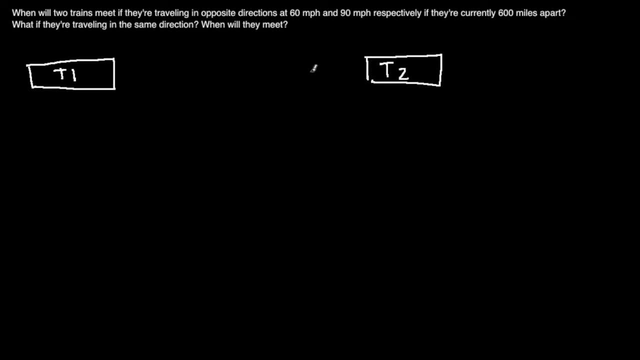 train 2.. So train 1 is traveling at a speed of 60 miles per hour and train 2 is traveling at a speed of 90 miles per hour. Train 2 is faster than train 1, so they're less likely to meet. 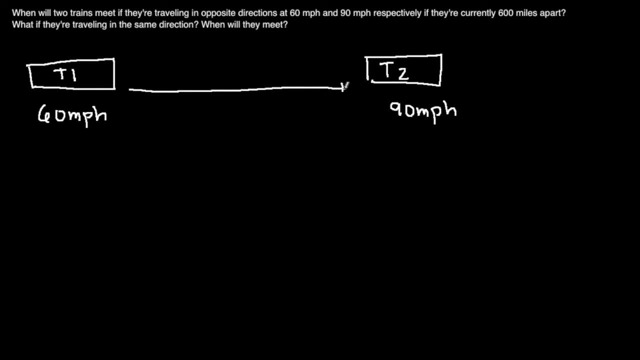 in the middle, So we have 600 miles apart And they're less likely to meet at the center because train 2 is traveling much faster than train 1, so they're probably going to meet somewhere around here. So the question is: when will they? 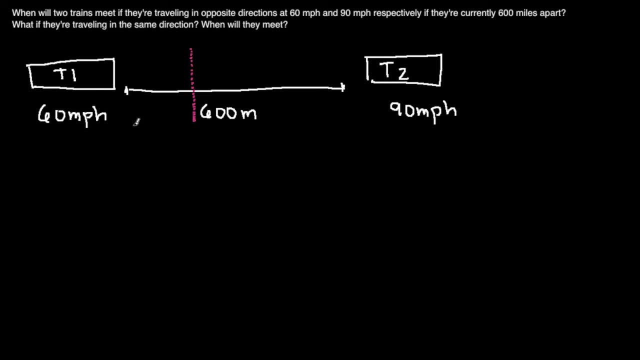 meet. We have to recognize that this is distance 1.. The amount of distance that train 1 has traveled, we will name it distance 1.. And the amount of distance that train 2 has traveled, we'll name it distance 2.. 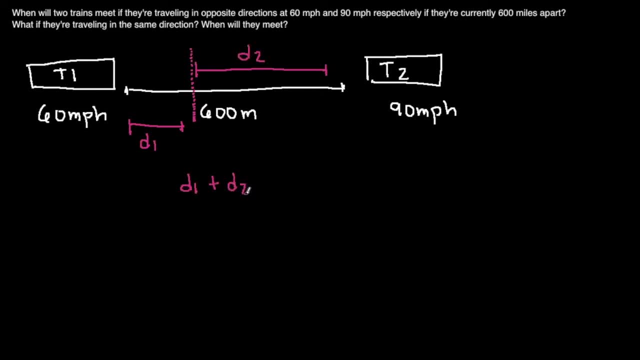 And we know that distance 1 plus distance 2 is equal to how far they are apart, which is 600 miles, Right? So we just have to come up with a formula that would give us their distance. And since they're traveling at a constant speed, 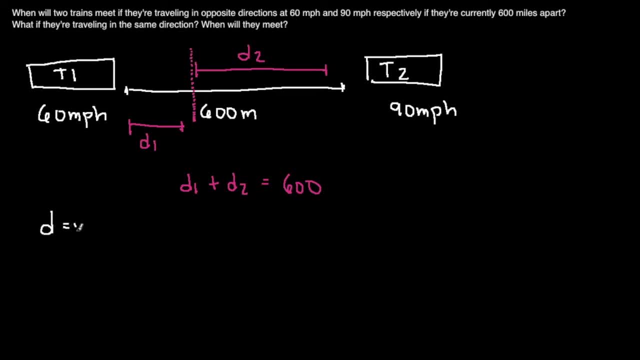 we only really just have to use: distance is equal to 60 times t, Alright, So we have. distance. 1 is equal to 60 times t, So we have 60t. And then for distance 2, we have for the second train. 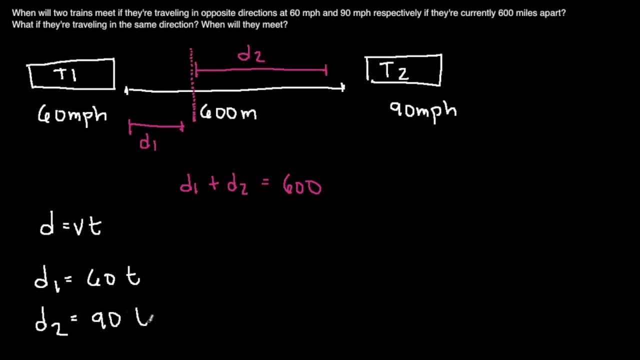 its velocity is 90 times t. So for distance 1 we have for the first train 60 miles per hour. That's its velocity times time. We don't have time yet. That's what we're looking for, So just leave it as it is. 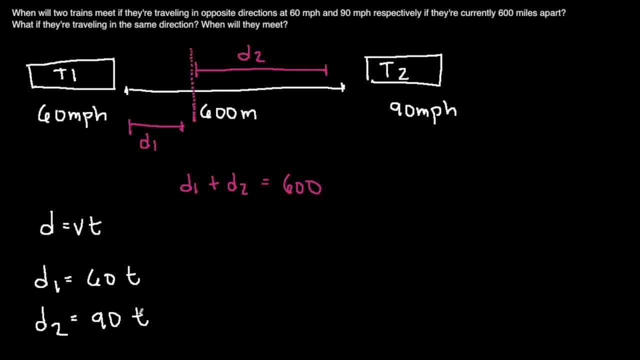 For distance 2 we have: velocity is 90 miles per hour times the time, which is t. So let's try to plug the equations that we made up to this equation. So we have: 60t plus 90t is equal to 600. 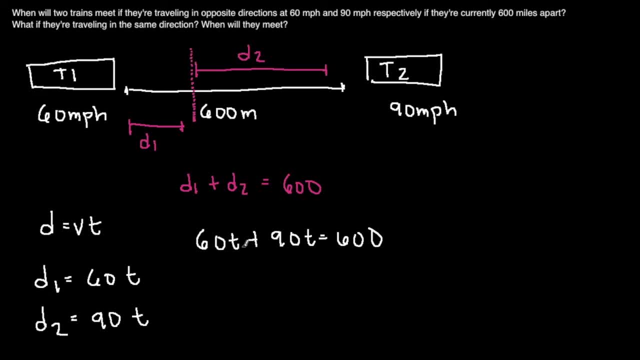 60 plus 90 is equal to 150 times t equals. I'm sorry, We have to make sure that the equal sign is in between the bar And we're going to divide both sides of the equation by 150 later on. So in order for us to find t, 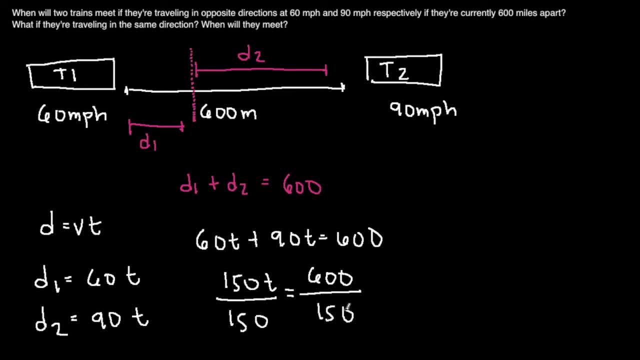 we have to divide both sides of the equation by 150.. Use division property of equality. So time should be equal to divided by 150, 4 seconds. So at 4 seconds it doesn't matter whether the distance is not equal if distance 1 is much smaller than distance. 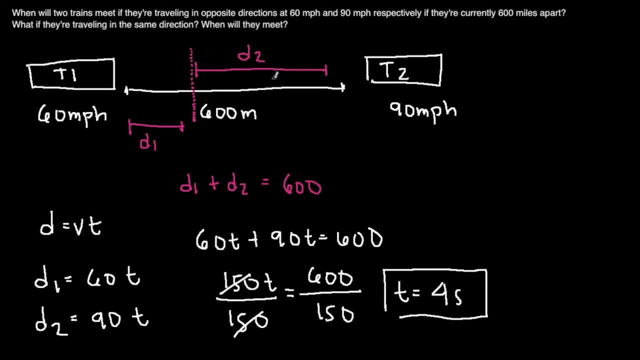 2 because, just like what I said, distance 2 or train 2 travels much faster, so it should travel a much larger distance than train 1.. It doesn't matter whether their distances are different. They will still meet at the same time, which is 4 seconds. 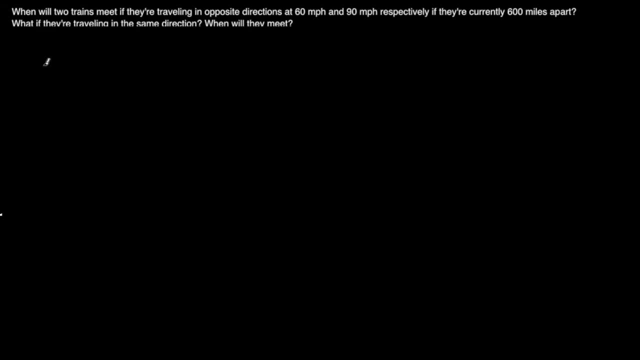 So for the second part of the problem we have: what if they're traveling in the same direction? So this is train 1 and this is train 2, and they still have 600 miles of a distance apart from each other. So in order for train 1 to 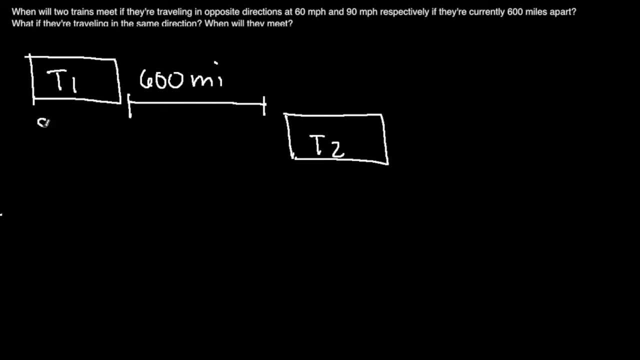 catch up with train 2, it should have the faster velocity. So this one should have 90 miles per hour and train 2 should have 60 miles per hour. It shouldn't be the other way around, because if train 2 travels faster than train 1, 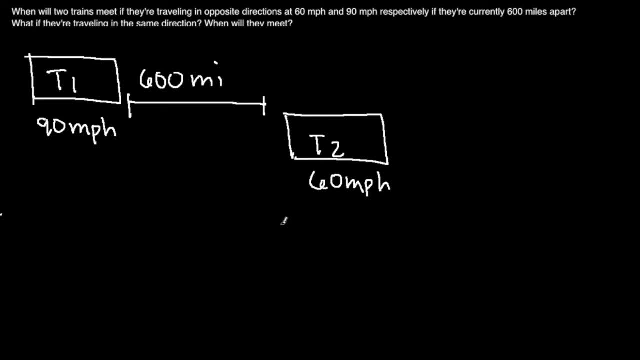 and it's already 600 miles further compared to train 1, then train 1 will never be able to catch up with train 2 if train 2 travels with a faster speed and it's 600 miles further before train 1.. At this point I'm going to introduce: 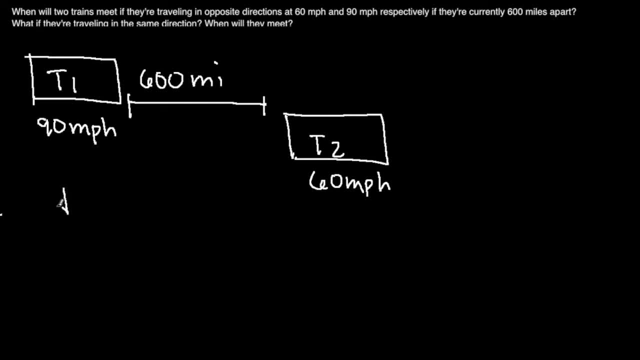 the relative velocity concept. We can solve this using relative velocity. It's equal to, d, is equal to v2 minus v1 or v1 times time 600. the distance apart is 600, v2 is 90 and v1 is 60. 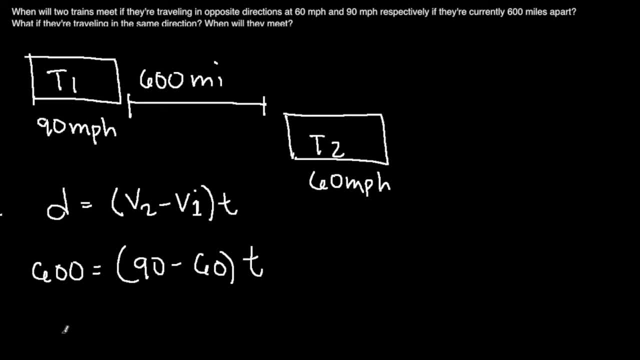 times time, So 600. so 90 minus 60 is 30, then we have 30 here. we divide both sides by 30 to get t, and t should be equal to 20 hours. Remember that we have hours here, It's not meters per second. 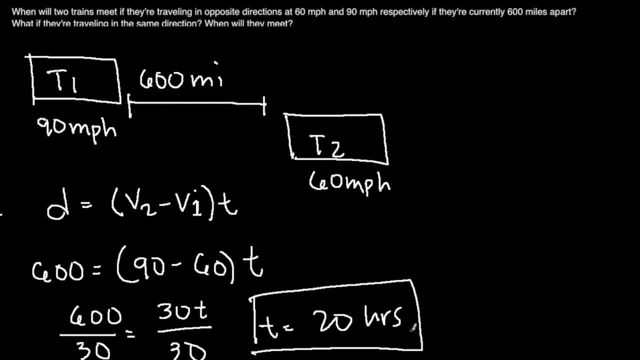 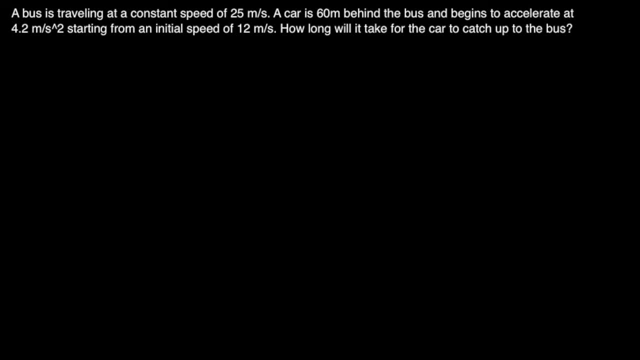 it's miles per hour, So our final answer for time should have the unit hours. A bus is traveling at a constant speed of 25 meters per second. A car is 60 meters behind the bus and begins to accelerate at 4.2. 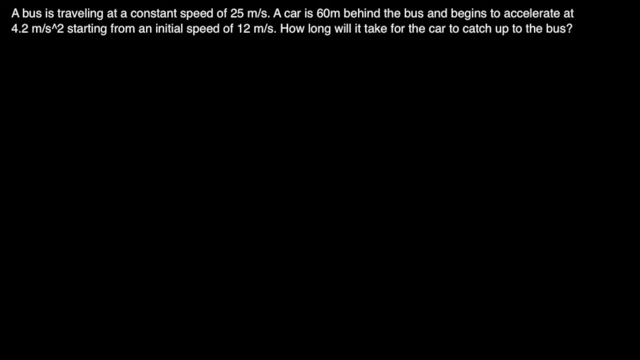 meters per second, squared. starting from an initial speed of 12 meters per second, How long will it take for the car to catch up to the bus? So let's try to draw a diagram with this situation. Let's say: this is the car, because the car is behind. 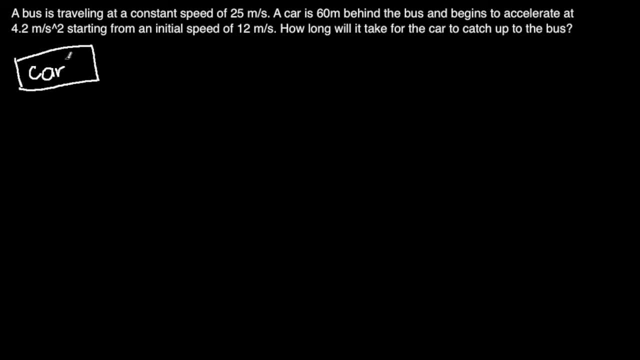 it And this is the bus. And they all start off at the same initial position, which is probably here. The car is 60 meters behind the bus. Let's try to draw that 60 meters. So this is the car and this is the bus. 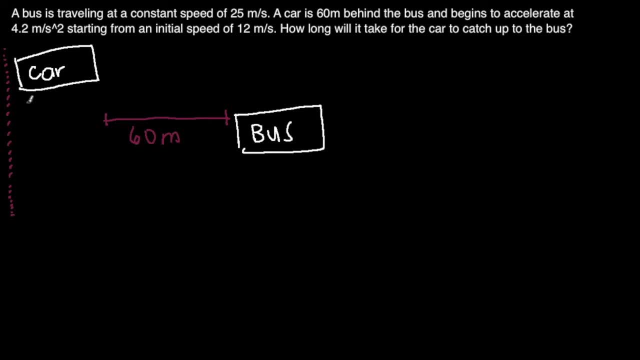 The car is traveling, It has an initial velocity of 12 meters per second and but it begins to catch up. it begins to accelerate so it can catch up with the bus. So it has an acceleration of 4.2 meters per second. squared. 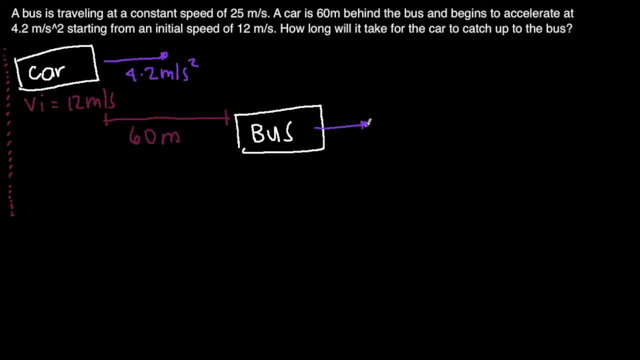 And we have the bus with a constant velocity, or a constant speed of 25 meters per second. Now the formula that we can use in order for us to express the distance of the car with respect to its acceleration is this: formula D is equal to. 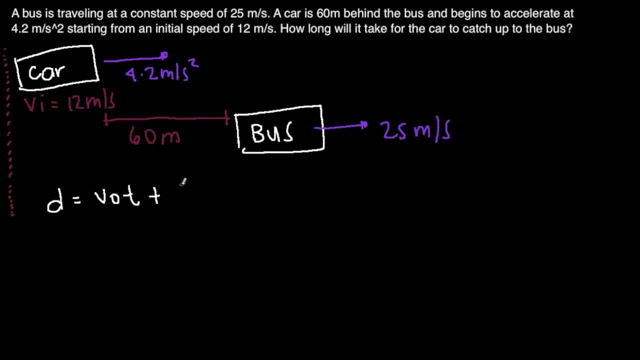 VOT plus one half of AT squared. Alright. So the displacement, because this is what it really is. D here stands for displacement. Now, displacement, remember, is the final position minus the initial position. So let's express D to this, to its real meaning. 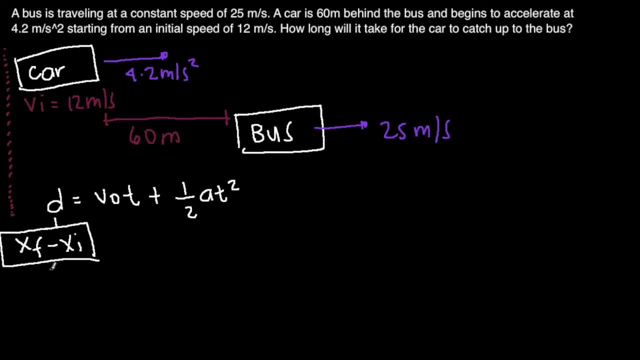 which is final position minus initial position. Remember that displacement means you have a final and initial position and it's the shortest distance from the initial to final. Now we will use that expression to this formula, So let's try to rewrite this into: XF minus XI. 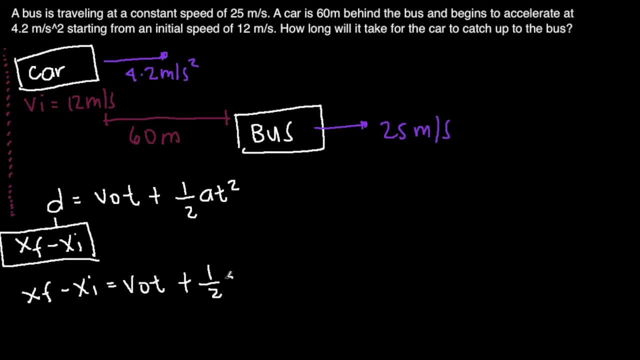 is equal to VOT plus one half AT squared, And we want to express this equation to the final position of the car. So let's transpose this and transfer this expression to the right and we will have: XF is equal to XI, or initial position plus VOT. 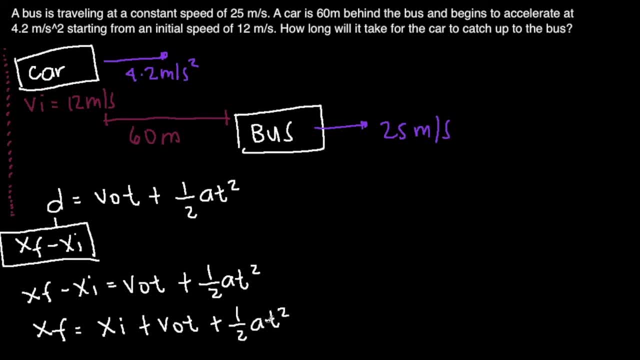 plus one half AT squared. The initial position of the car is zero because it starts off from the origin from where both of the vehicles start, which is at zero meters. Remember it's here. So all we really have is zero. So let's cancel this. 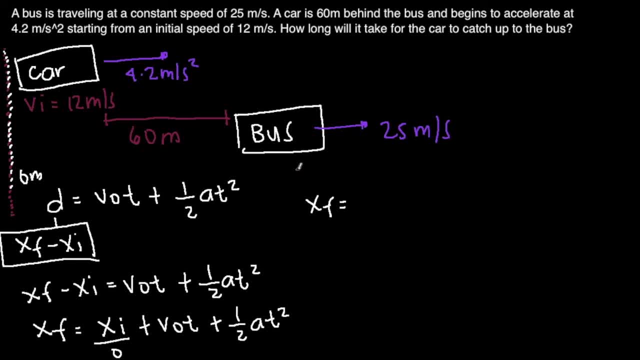 This is going to be zero. This is going to be gone for the car. Let me write it here. So all we really have is initial position or initial velocity. is we have 12 times the time, which is what we're looking for, because we want to know how long? 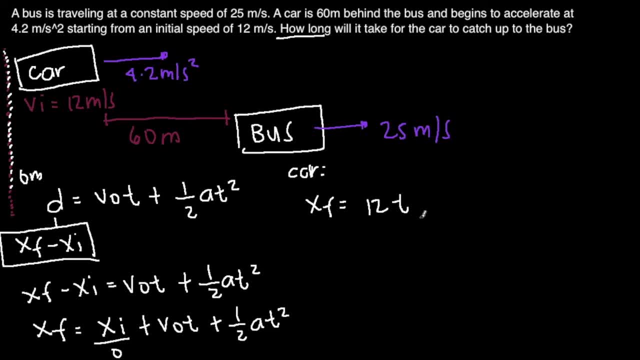 it will take for both to catch up to each other. And then we have plus one half of acceleration, which is 4.2 T squared. Now, one half or 4.2 is 2.1.. So let's try to simplify this. 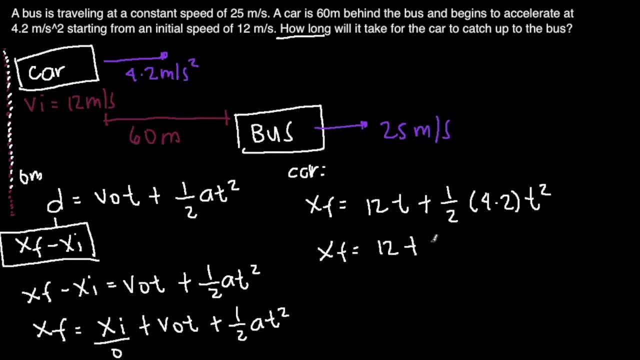 expression. We have 12 plus 2.1 T squared, So we can get the final position of the car using this expression at any time. Just plug in the time whatever time it is. For example, if you want to know the final position of the car at 5 seconds. 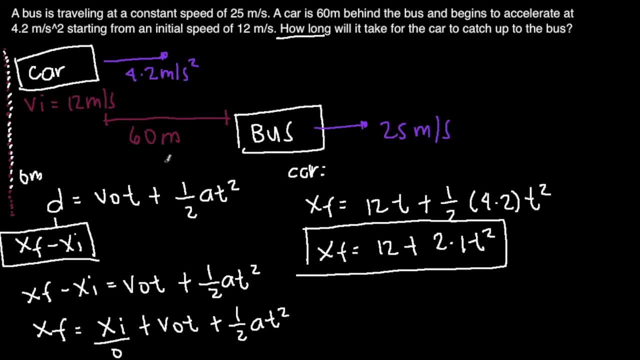 just plug it in here and you can find the final position of the car with respect to its initial position, its acceleration and initial velocity. Now, this is for the car. Let's find this expression for the bus. So we have final position. this is for the bus. 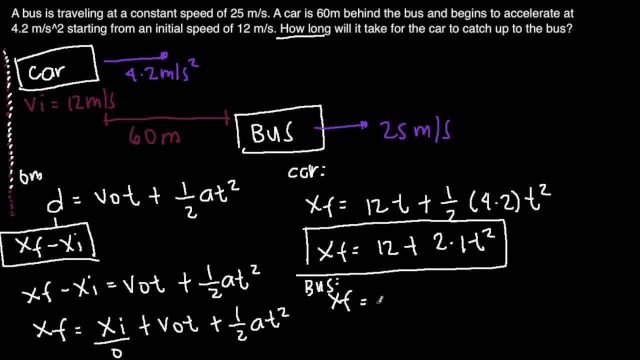 we have final position and then initial position is going to be 60, because it's already 60 meters ahead of the car. So we put 60 here for the initial position, plus the initial speed is 25 T and then it doesn't have any. 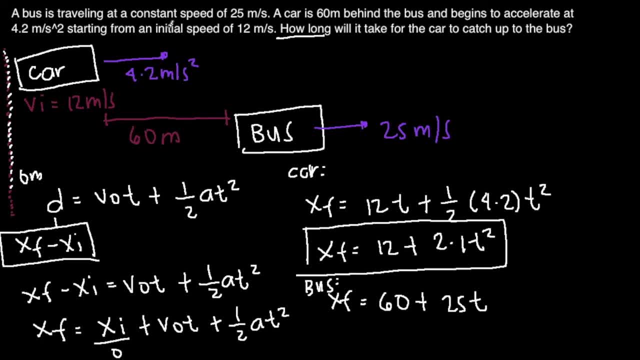 acceleration. Remember the car- I mean the bus- is traveling at a constant speed, so it doesn't have any acceleration. This term goes away, So all it really has is 60 plus 25 T, So this is what we're going to use for. 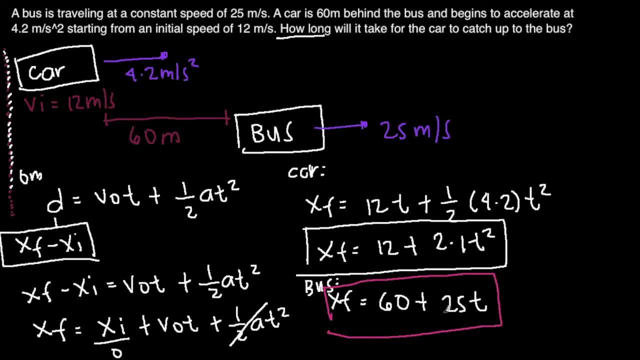 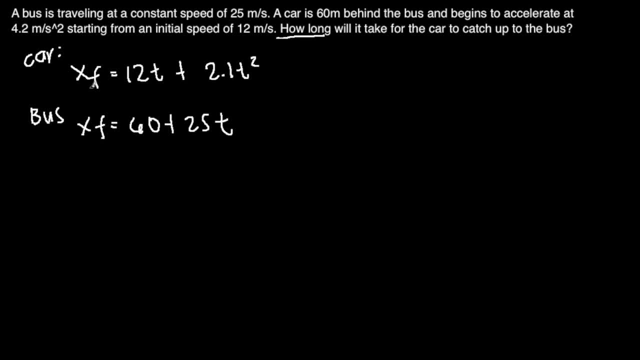 determining the position of the bus at any time with respect to its initial position, which is 60.. Okay, so the next thing that we do after we get the expressions for the final position of both the car and the bus, is we put both of the expressions or the equations. 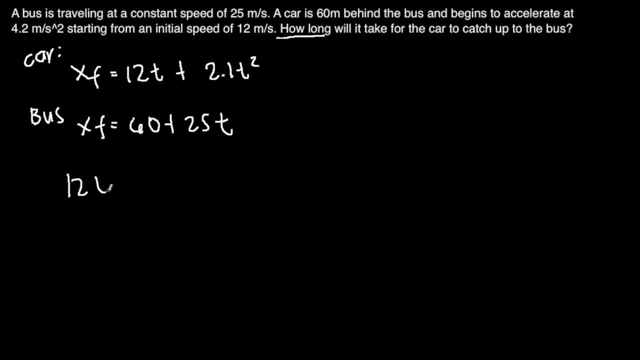 equal to each other. So we have 12 T plus 2.1 T squared equals 60 plus 25 T. So what I want to do is I want to transfer all of the terms to the left, So we have 2.1. 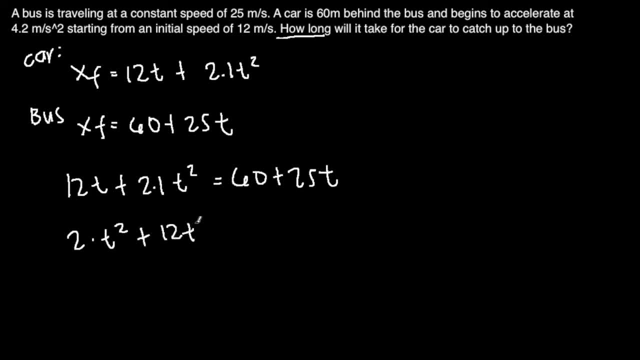 T squared plus 12, T minus 25, T minus 60 equals 0.. So let's simplify even further: 12 minus 25 is equal to negative 13.. So we have 2.1. I mean, uh, 2.1. this should be 2.1. 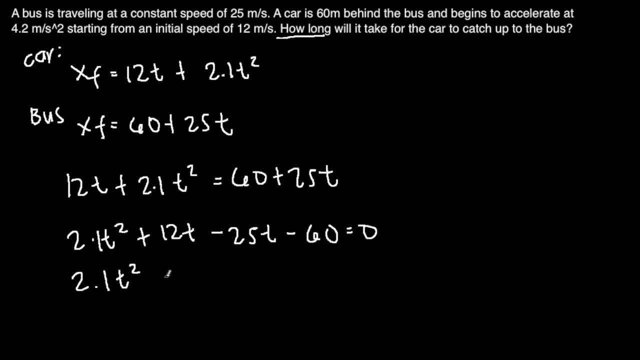 2.1. T squared minus 13, T minus 60 equals 0.. So, in order for us to find the time or the variable, notice that we have a quadratic equation. Whenever you have a quadratic equation and you want to extract the variable. 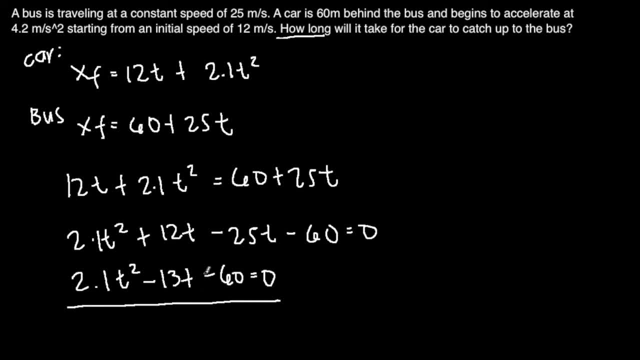 it's best to use a quadratic formula Whenever you have an equation with an expression of AX squared plus BX plus C equals 0, that's what you call a quadratic equation. So it's in this format: X squared plus X plus C is equal to 0.. 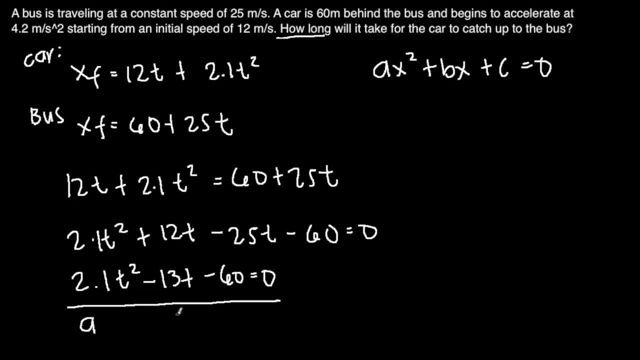 Notice that this is our A, this is our B and this is our C. So we just have to plug in these values into our quadratic formula. And this is our quadratic formula. T is equal to negative of B plus minus square root of B squared. 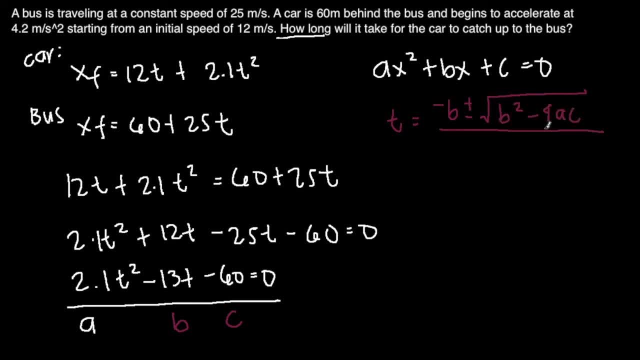 minus 4AC all over 2A, So you just have to plug in the values for A, B and C. I already labeled it for your convenience. So we have: T is equal to B is negative 13, so it will become positive 13. 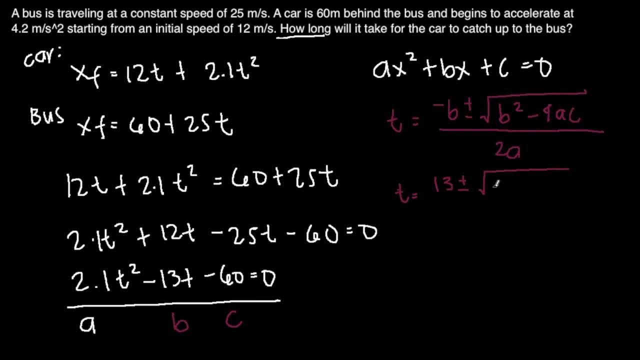 plus minus square root of negative 13 squared minus 4, A is 2.1, C is negative 60, all over 2 times 2.1. So all we really have to do is plug it into our calculators and let's see what the value is.